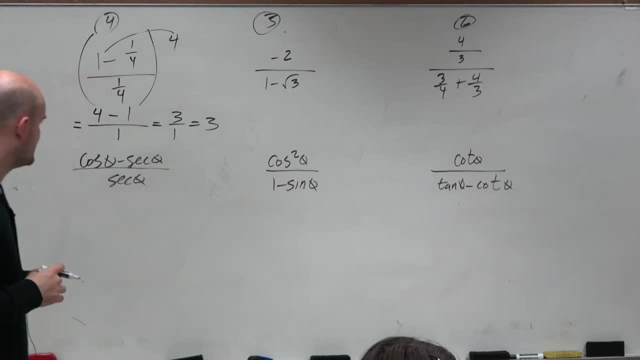 If our goal- technically our goal here is Our goal here- is to multiply by the number of fractions inside of our larger fraction, Our goal here is to get this Since our since we only have one fraction in the denominator. we know this problem will be a lot easier if this is one Agreed Right, So why don't? 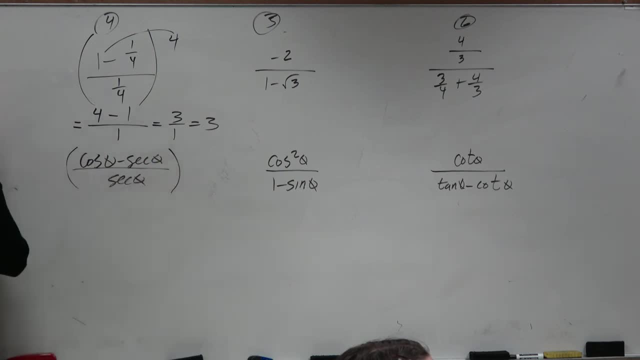 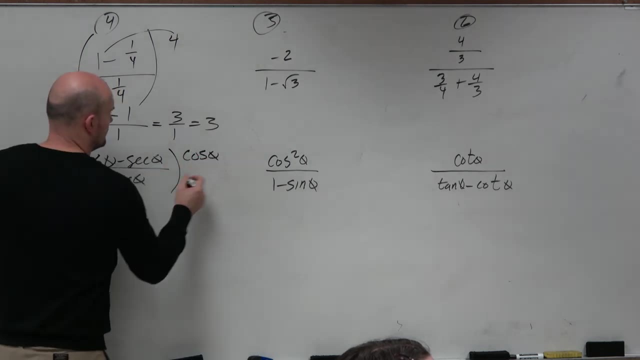 we just multiply everything times. the reciprocal of that denominator, which is this reciprocal of secant, is cosine, Which, again, guys, if you write these, that's one over cosine, that's one over cosine, right, And that's one. So again, this would be reciprocal. So in this, 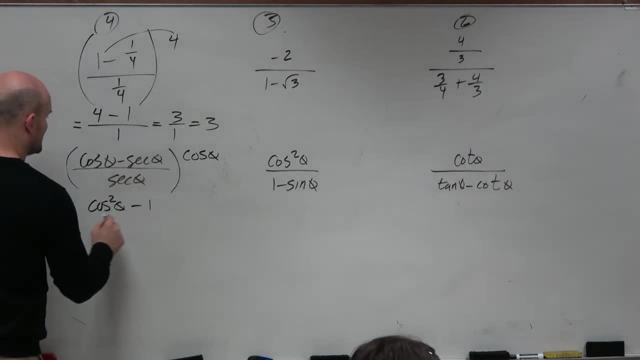 case we get cosine squared Of theta minus one all over one, which you don't really need to write the one in the denominator, but you know it's there And we recognize. cosine squared of theta minus one is Pythagorean identity. Nope, still forgot it. Okay, let's do it again: Cessin squared. 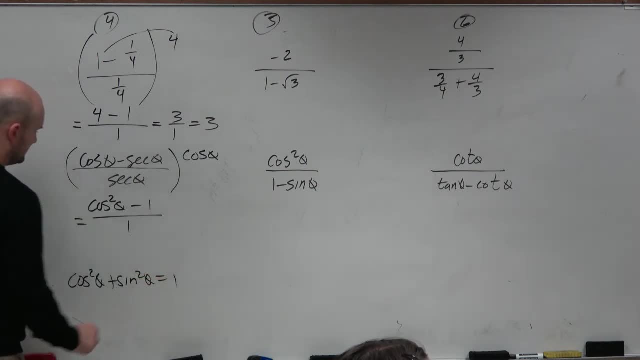 of theta plus sine squared of theta equals one. So if I subtract a one to give me cosine squared of theta minus one, I would need to subtract the sine squared. So therefore this is equal to Negative, Negative, Negative. 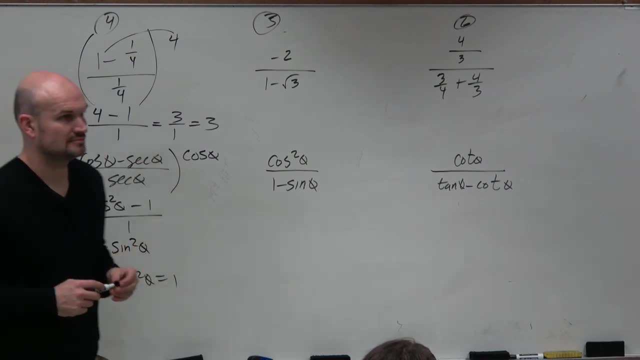 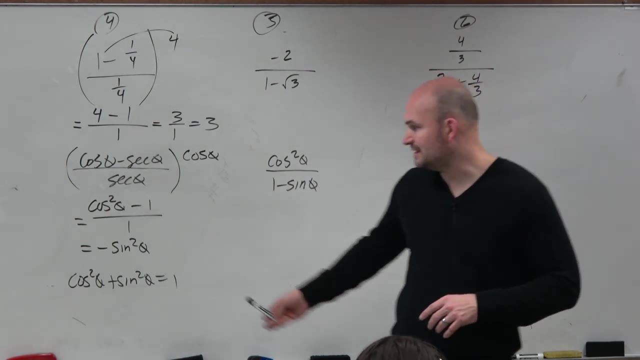 Negative sine squared of theta. Do you guys see why it's a negative sine squared, not a positive sine squared? Yes, So we need to know this, and we just need to make sure we know how to manipulate it as well. Next round: 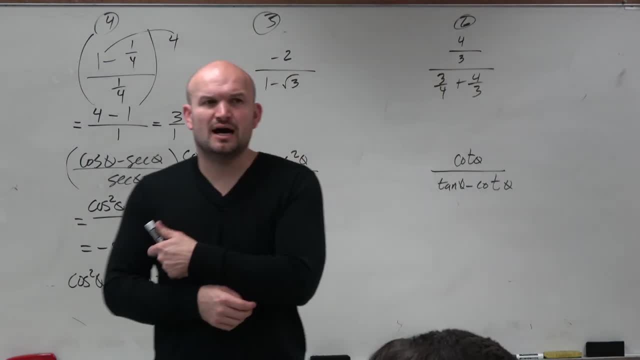 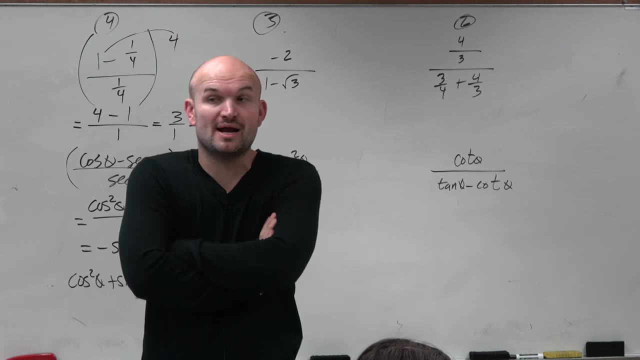 Now this one. we don't really have any fractions, but we have a radical in the denominator And on the what you need to know, I gave you before break. I told you to rationalize those. We're going to practice rationalizing. 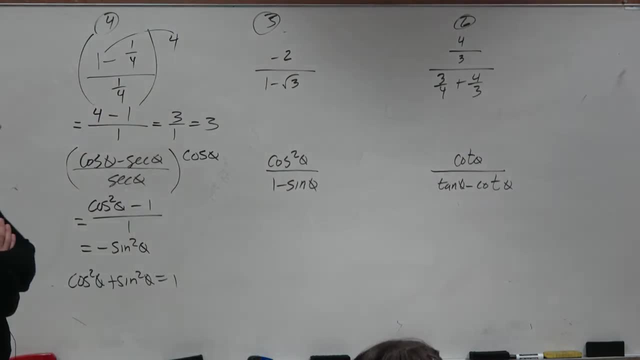 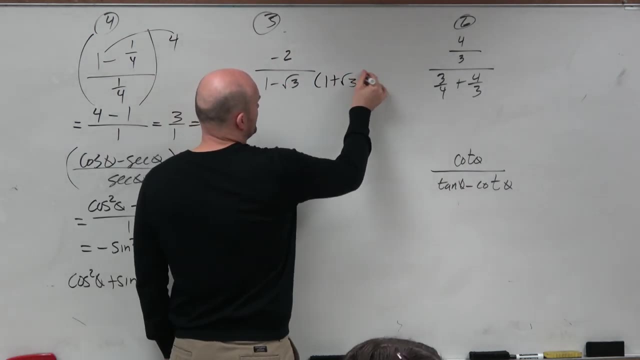 So if I wanted to get rid of the radical in this case, I would need to rationalize the denominator, which would be multiplied by the conjugate. So the conjugate of 1 minus the square root of 3 is 1 plus the square root of 3.. 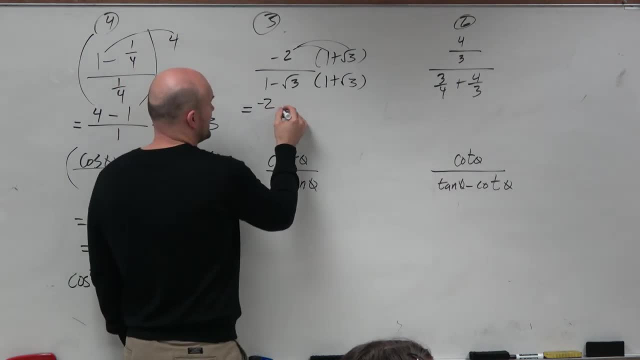 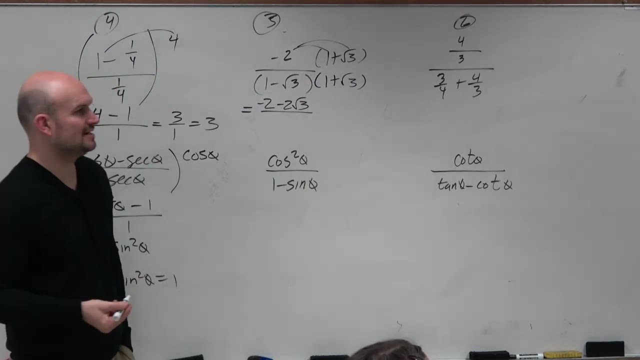 And the nice thing about rationalizing the denominator is: here we get negative 2 minus 2 square root of 3. Here we have a difference of two squares. Wow, we're practicing that a lot. I wonder if this will come up later. 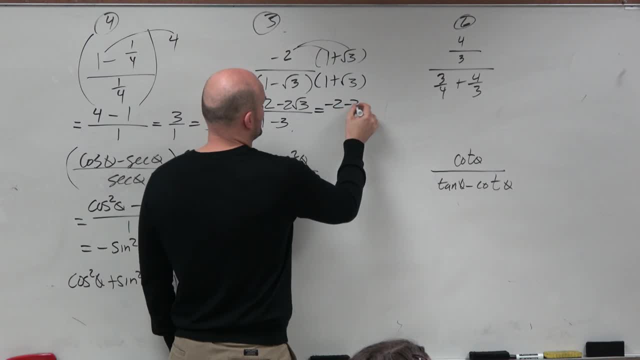 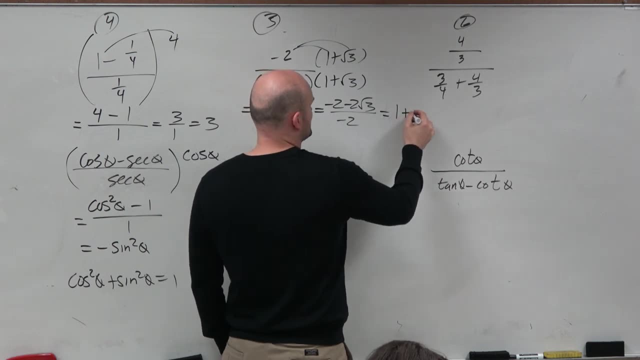 It will, don't worry. So that simplifies to negative 2 minus 2 square root of 3 divided by negative 2.. The negative 2 divides into both those terms, which gives us a 1 plus the square root of 3.. 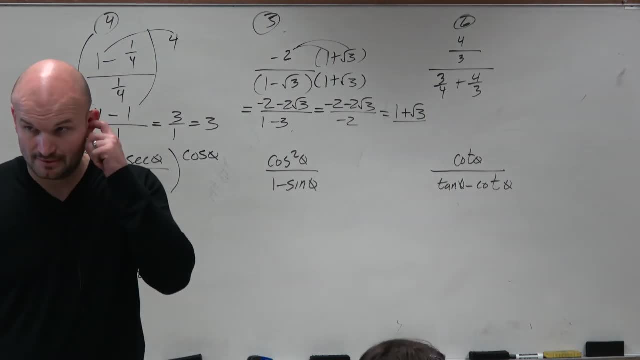 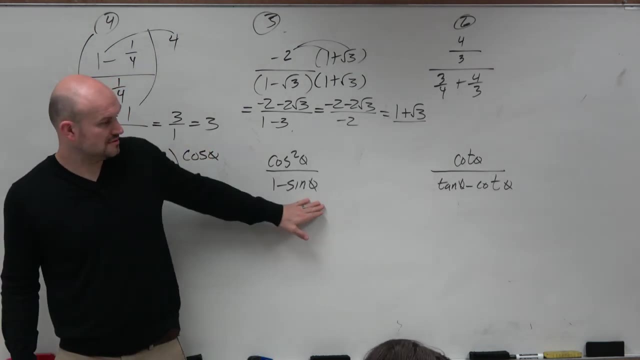 And don't worry guys, we will be doing that later this chapter. All right, but you guys can see the algebra that just happened. Practice it. So here, maybe I want to multiply by the conjugate here: What's the conjugate of 1 minus sine? 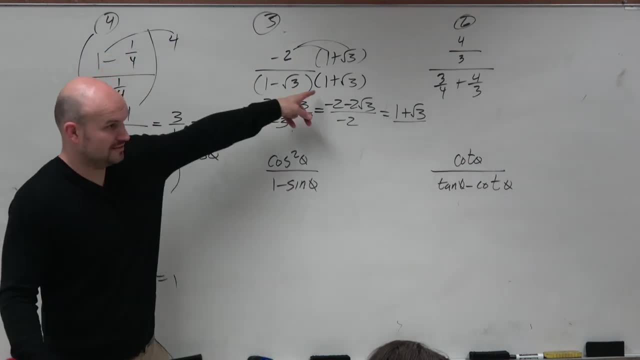 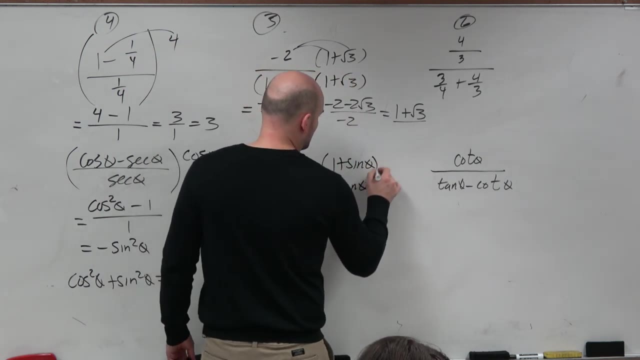 1 plus sine, just like over here. So what happens here? I don't know, Let's try it. Remember when I said to just try things. Maybe you get it wrong, Maybe it doesn't work, Try something else. The nice thing about multiplying by its conjugate. 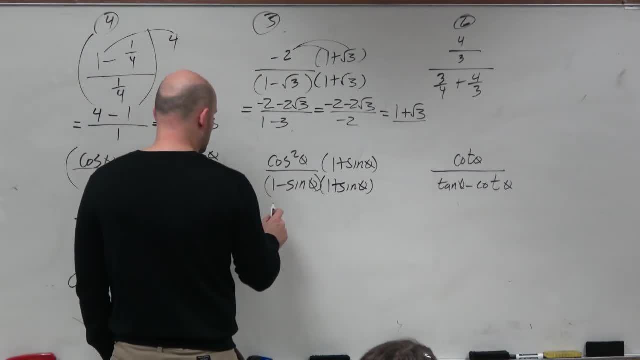 is we get the difference of two squares. So up top we're left with cosine squared of theta times 1 plus sine of theta. I could distribute that, but I'm just going to leave it right now. This becomes 1 minus sine squared of theta. 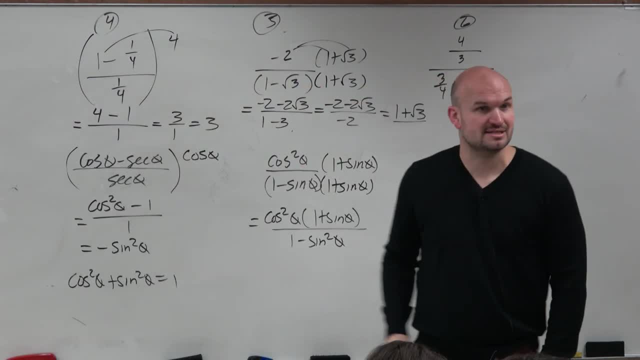 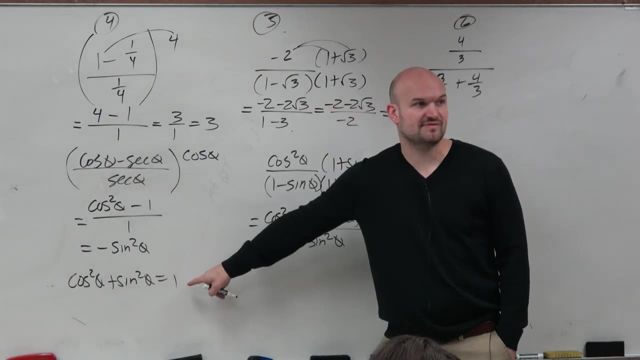 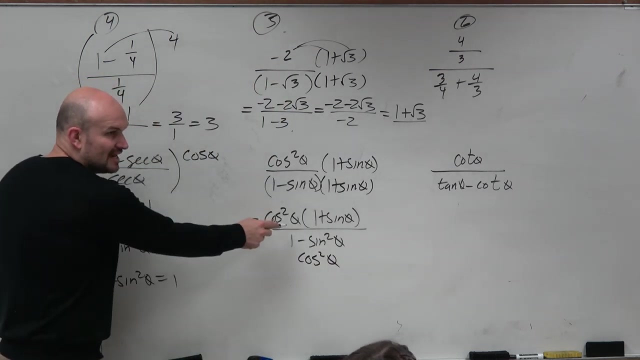 Sine squared of theta. Do we recognize anything special about 1 minus sine squared of theta? What does that equal to? 1 minus sine squared of theta is the same thing as cosine squared of theta? Hey, I have a cosine squared of theta in the numerator. 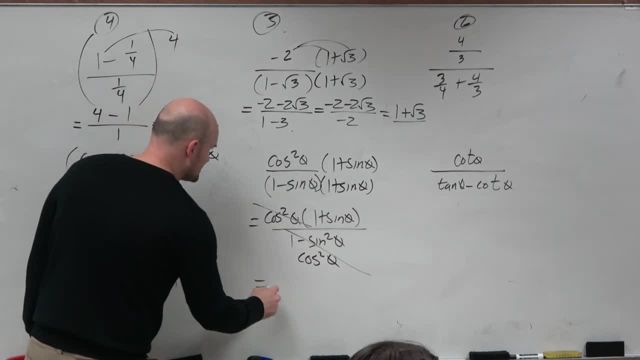 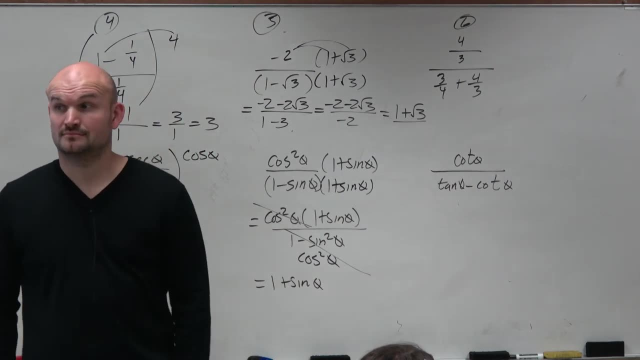 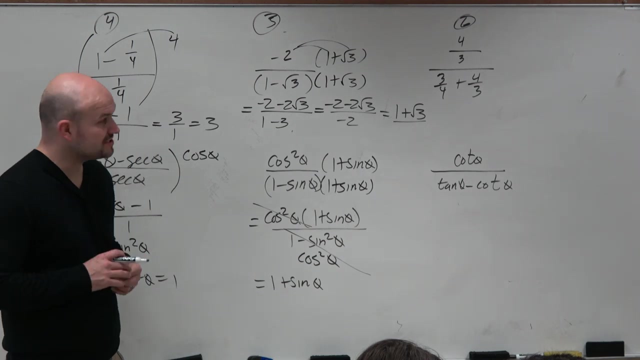 as well as in the denominator That divides out. That just leaves me with 1 plus the sine of theta. All right, Last but not least, now again we have multiple fractions in this case, So again we want to identify the LCD. 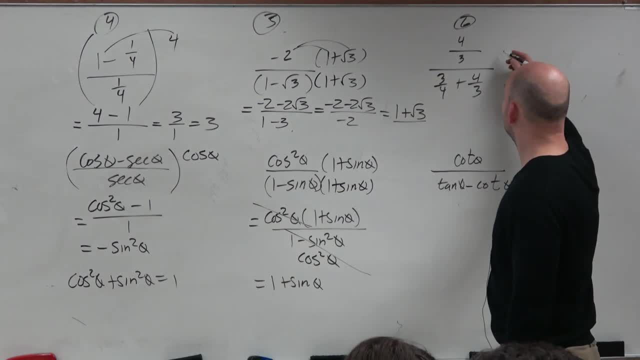 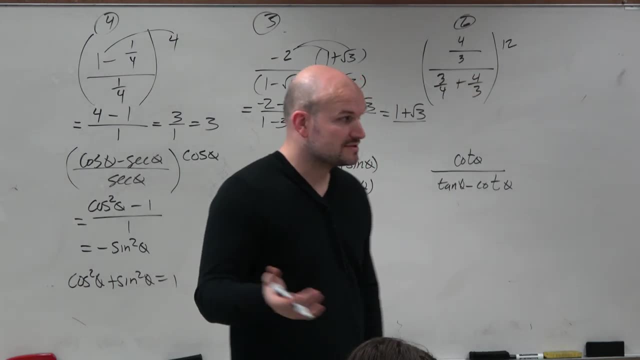 We could say: it's going to be 3 times 4 is going to be 12.. So let's multiply everything times 12.. You could also multiply by the conjugate, kind of see where that goes, And now you might not recognize. well, oh, let's actually. 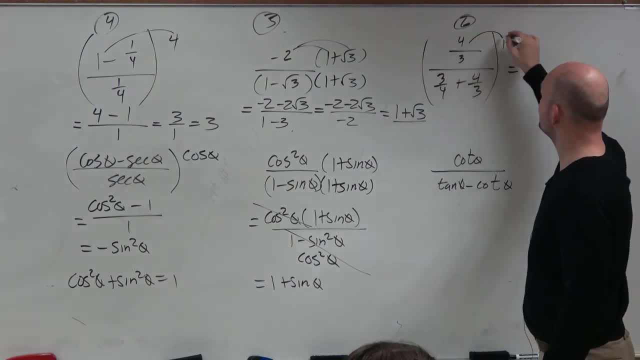 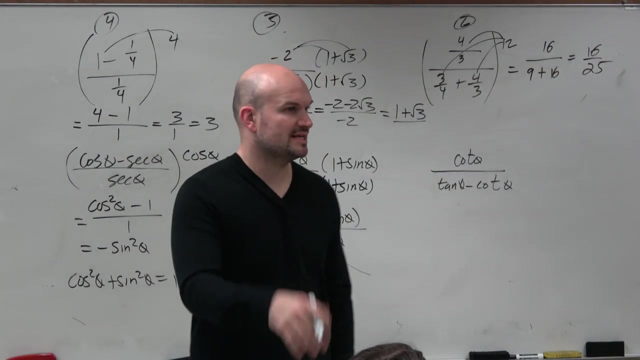 do this real quick, sorry. So if I were to multiply everything times 12, I would get 16 over 9 plus 16, which equals 16 over 25.. So again you can see how multiplying by the LCD helps us there.